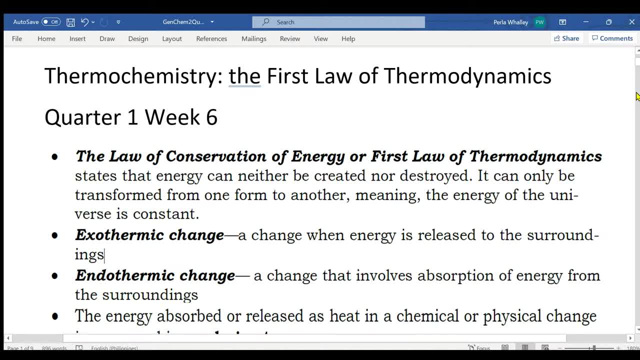 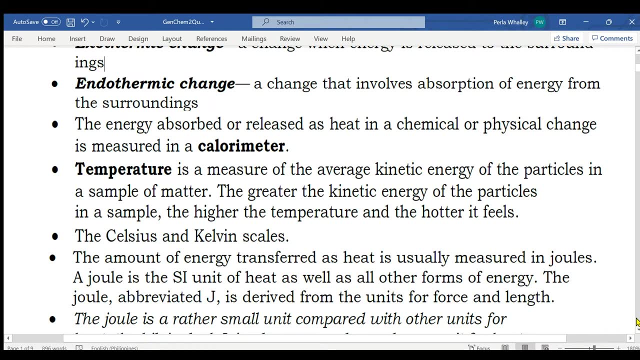 Endothermic Change, a change that involves absorption of energy from the surroundings. Example: photosynthesis. The energy absorbed or released as heat in a chemical or physical change is measured in a calorimeter. Temperature is a measure of the average kinetic energy of the particles in a sample of matter. 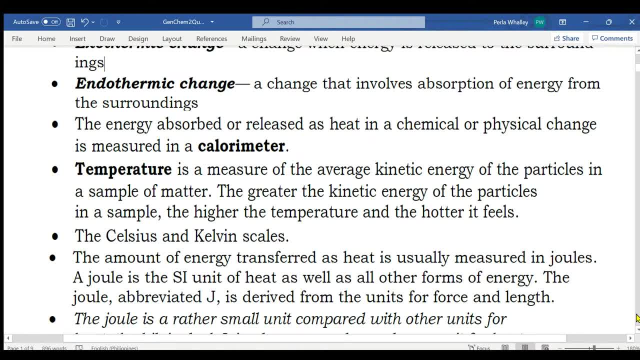 The greater the kinetic energy of the particles in a sample, the higher the temperature and the hotter it feels. The Celsius and Kelvin are the unit used for temperature. The amount of energy transferred as heat is usually measured in Joules. A joule is the SI unit of heat as well as all other forms of energy. 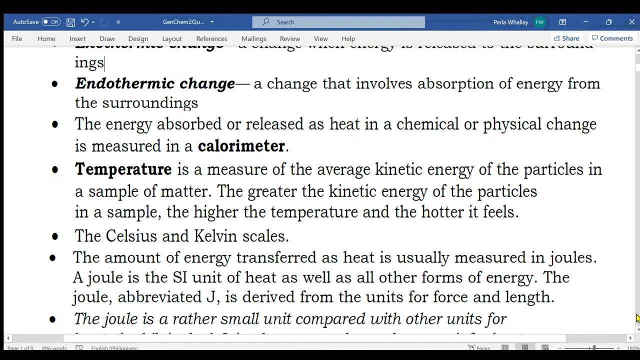 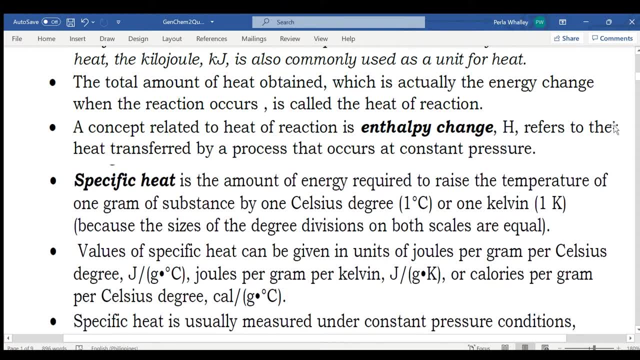 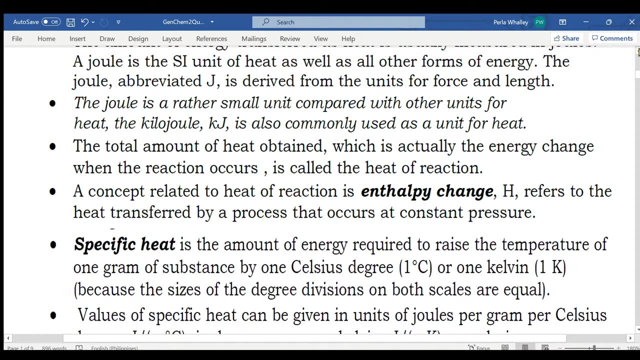 The joule, abbreviated as capital letter J, is derived from the units of force and length. The joule is a rather small unit compared with other units for heat. the kilojoules, or kJ, is also commonly used as a unit for heat. 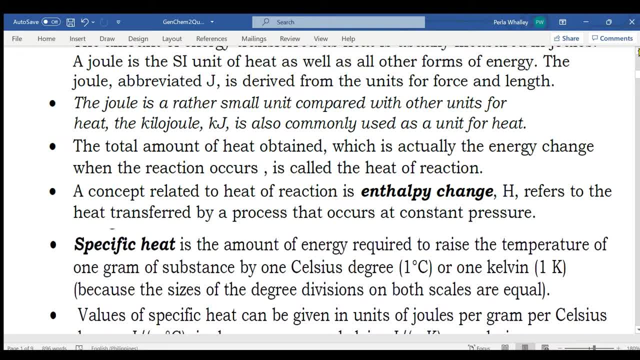 The total amount of heat obtained, which is actually the energy change when the reaction occurs, is called the heat of reaction, a concept related to heat of reaction as enthalpy change. H refers to the heat transferred by a process that occurs at constant pressure. 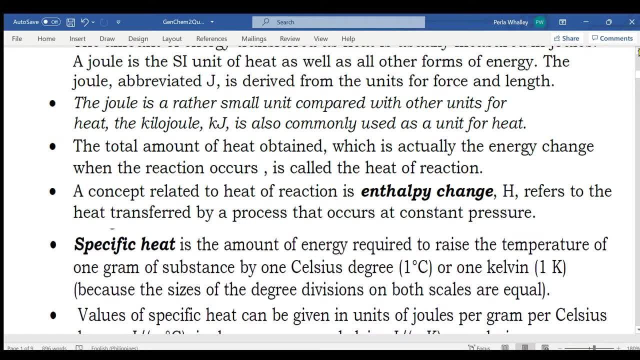 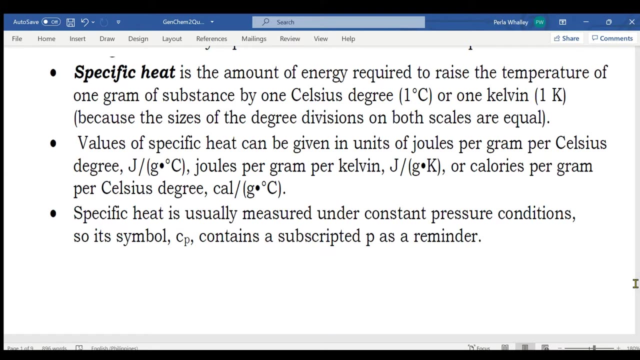 Specific heat is the amount of energy required to raise the temperature of one gram of substance by one Celsius degree or one Kelvin. because the sizes of the degree diversions on both scales are equal, values of specific heat can be given in units of Joules per gram per. 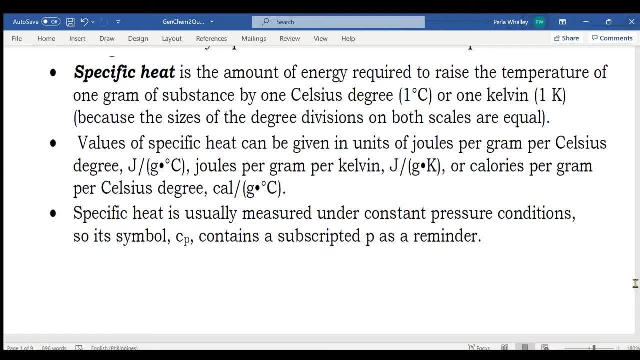 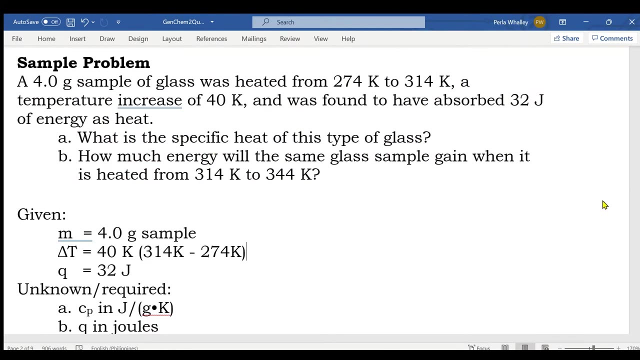 Celsius degree, Joules per gram per Kelvin or calories per gram per Celsius degree. specific heat is usually measured under constant pressure conditions, so its symbol is C. sub P contains a subscripted P as a reminder. sample problem: a four point series sample of glass was heated from 274 to 314 Kelvin. a temperature increase of 40 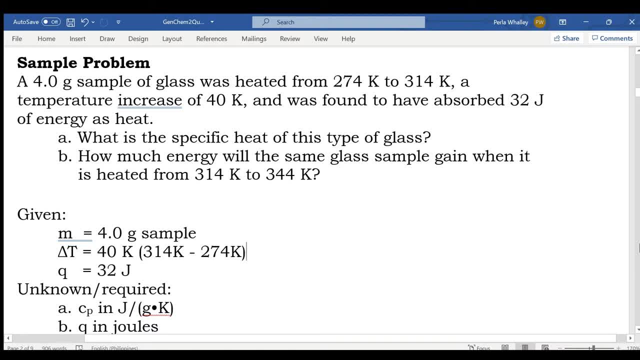 Kelvin and was found to have absorbed 32 Joules of energy as heat. what is the specific heat of this type of glass and how much energy will the same glass sample gain when it is heated from 314 to 344 Kelvin? again, we have to write the. given the unknown order required, the formula and the. 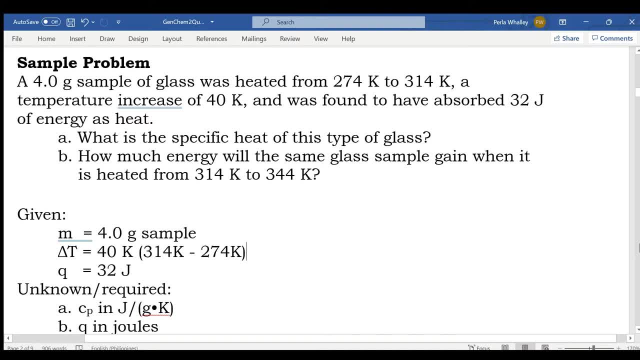 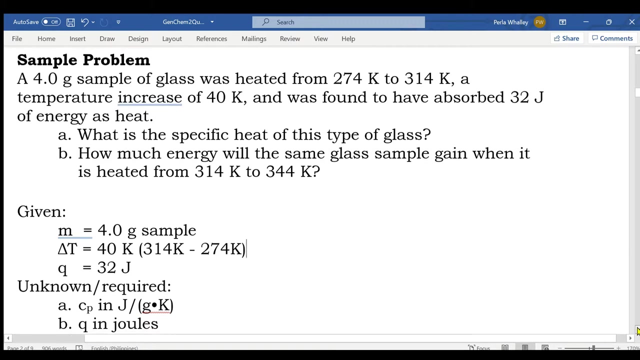 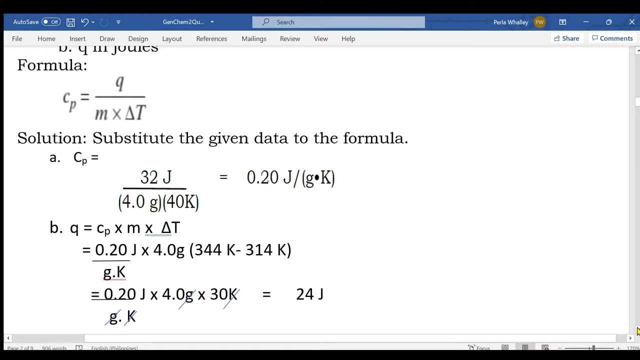 solution given as the four grams of sample and the change in temperature as equal to 40 Kelvin and Q, or heat is equal to 30 Joules, unknown CP and Joules per gram times Kelvin and Q and Joules. so the formula: CP is the specific heat at constant pressure, Q is the heat, M as 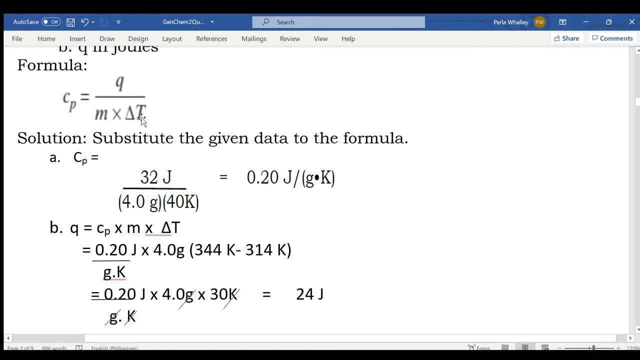 the mass and Delta T is the change in temperature. we have those values and what we need now is substitute the given data to the formula. so Q is 32 Joules divided by the mass, which is four point zero grams times 40 Kelvin. so dividing this is equal to 0.20 joules per gram times Kelvin. joules per gram times Kelvin. next, heat: 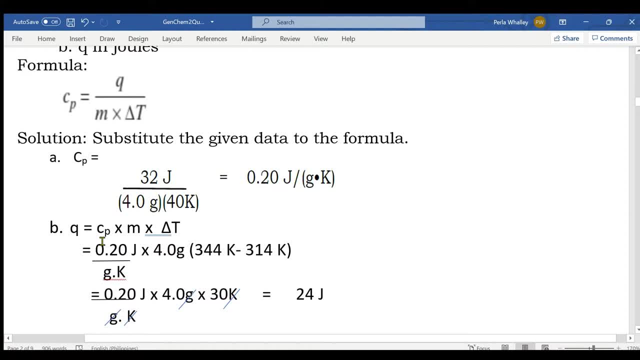 is equal to the specific heat at constant pressure times, mass times the Delta T. how did we have that formula? that is, we derive it by cross multiplying. okay, so Q is equal to C P times M times Delta T. so C P is equal to 0.20 joules gram times Kelvin times the mass, which is 4.0. 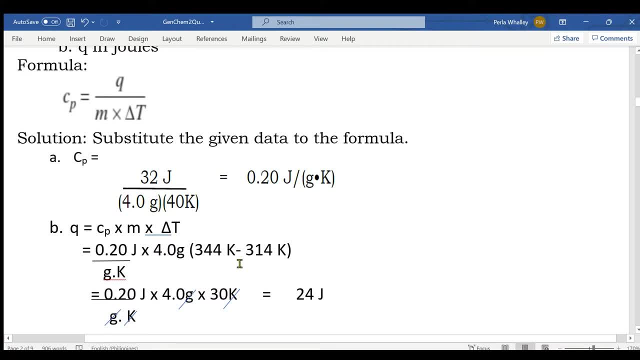 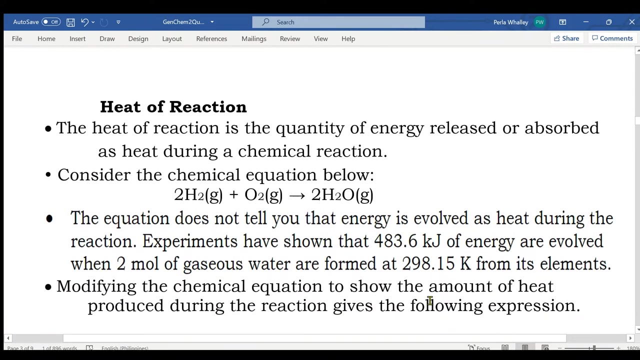 grams times the Delta T, T, which is equal to 30. so grams and grams concept, Kelvin and Kelvin concept, and the answer is 24 joules. let's go now to head of reaction. the head of reaction is the quantity of energy released or absorbed as heat. country水: 0.25, a select quantity here. don't forget to check out levels and values and all other parameters if you want to read the cash check, the yo-yo SC. 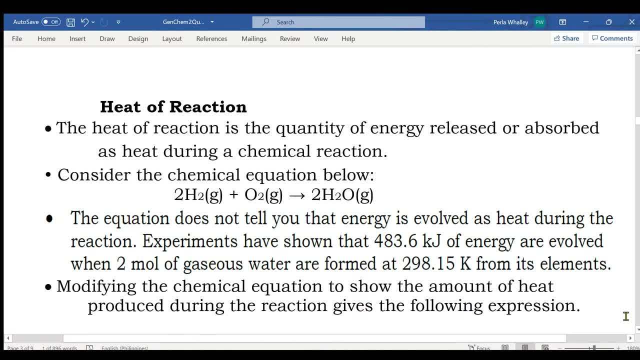 during a chemical reaction. consider the chemical equation below: two moles of hydrogen gas plus one mole of oxygen gas will form two moles of water in gaseous form. water in gaseous form is vapor. the equation does not tell you that energy is evolved as heat during the reaction experiments. 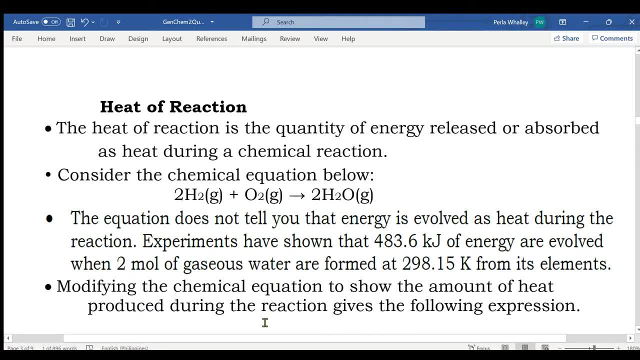 have shown that four hundred eighty three point six kilojoules of energy are evolved or released. when two moles of gaseous water was formed at two hundred ninety eight point one, five Kelvin from its elements, modifying the chemical equation to show the amount of hydrogen gas formed in gaseous form will be one mole plus one, mole of hydrogen gas plus one. 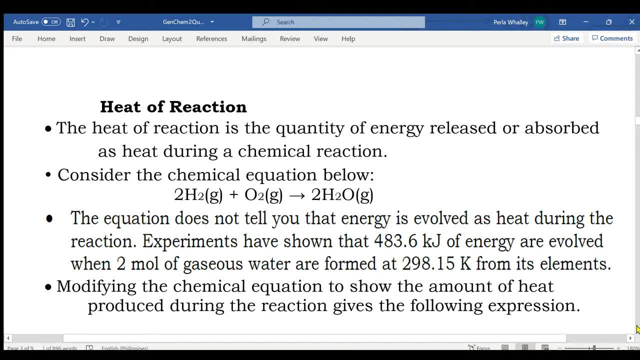 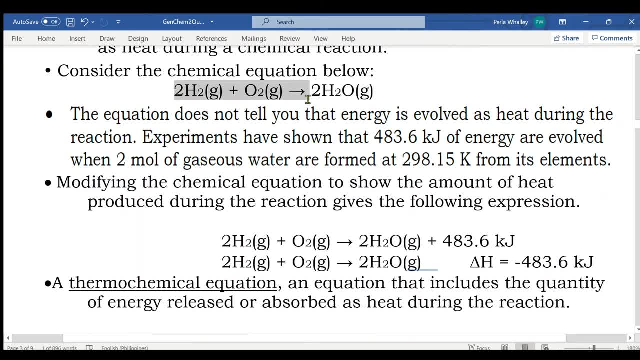 of heat produced during the reaction gives the following expression: so from this equation we can now add four hundred eighty three point six kilojoules of energy evolved or released. when it is evolved or released, that means the energy should be placed in the reactant site. so we can. 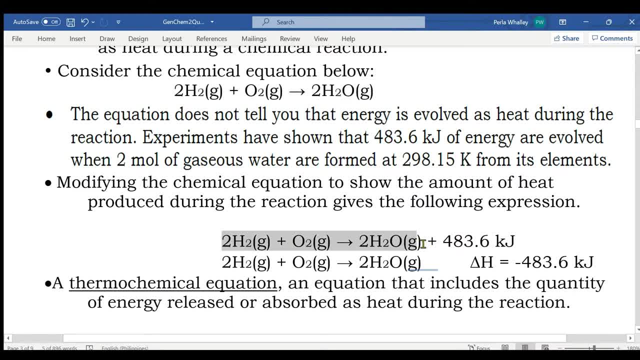 rewrite it as this: one: okay, plus four hundred eighty three point six kilojoules of energy evolved or released, okay. or it can also be rewritten like this: that means that the energy evolved or released is not included in the formula. but you can write it as: Delta H is equal to four hundred eighty three point six kilojoules, but 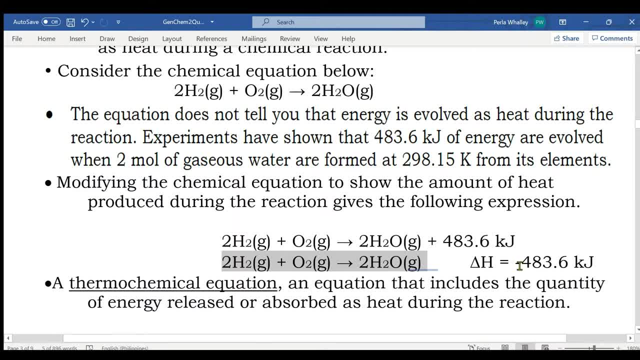 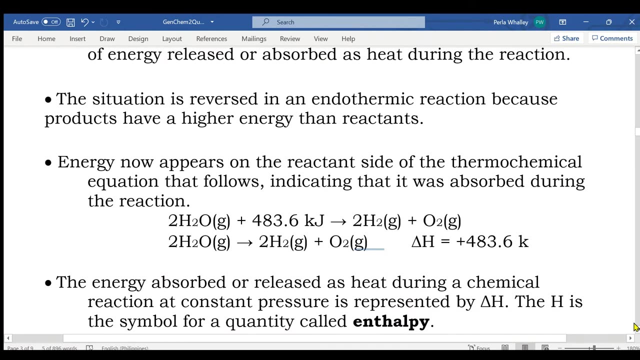 it is negative because it is evolved or released. a thermochemistry. the thermochemical equation, is an equation that includes the quantity of energy released or absorbed as heat during reaction. the situation is reversed in an endothermic reaction, because products have a higher energy than reactants. energy now appears on the reactant side of a. 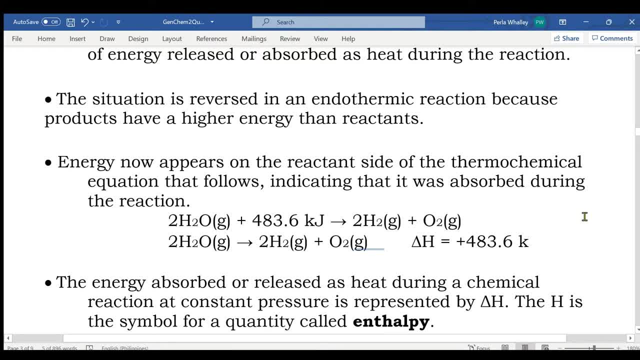 thermochemical equation that follows, indicating that it was absorbed during the reaction. when it is absorbed during the reaction, it is added, and the reactant side, or it can be also expressed as this, which is not included, and the reaction. but you have to write Delta H is equal to. 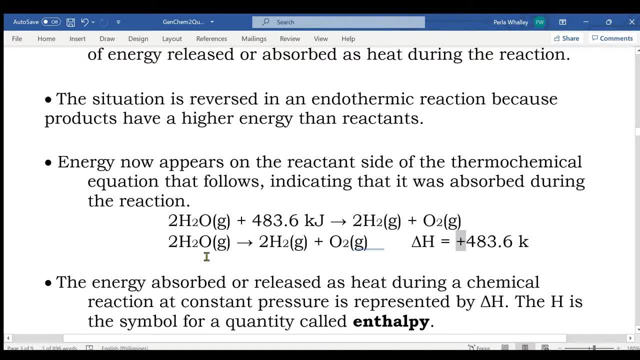 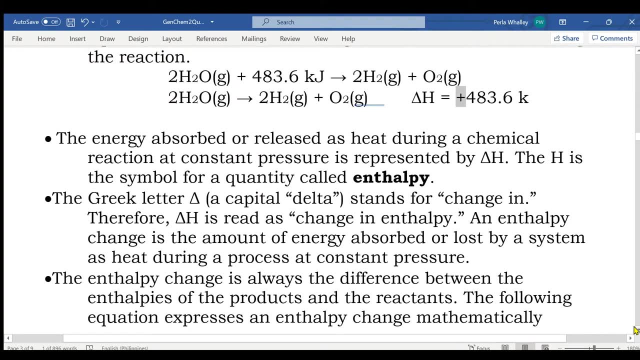 positive because it is absorbed. the energy absorbed or released as heat during a chemical reaction at constant pressure is released and the reaction is added. and the reaction is absorbed as heat during a process at constant pressure is released and the reaction is represented by Delta H. the H is the symbol for a quantity called enthalpy. the Greek letter Delta, a capital Delta, stands for 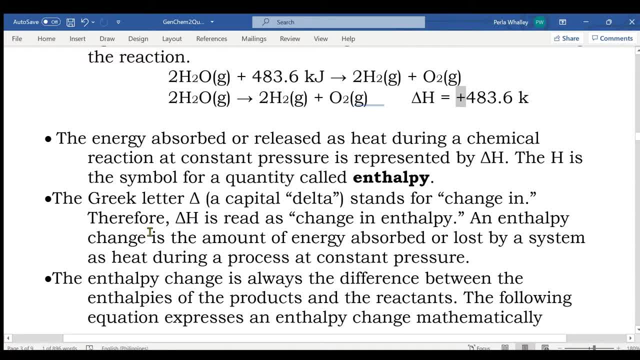 change in. therefore, Delta H is read as change in enthalpy. an enthalpy change is the amount of energy absorbed or lost by a system as heat during a process at constant pressure. the enthalpy change is always the difference between the enthalpies of the products and the 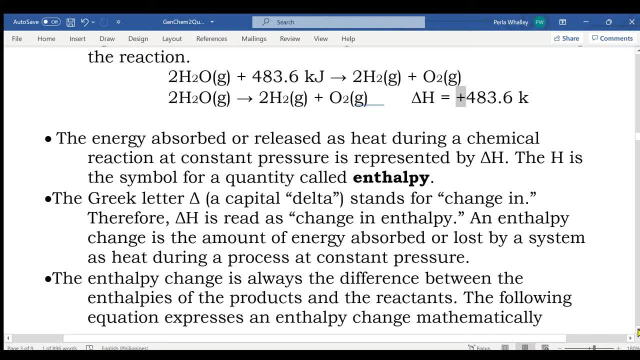 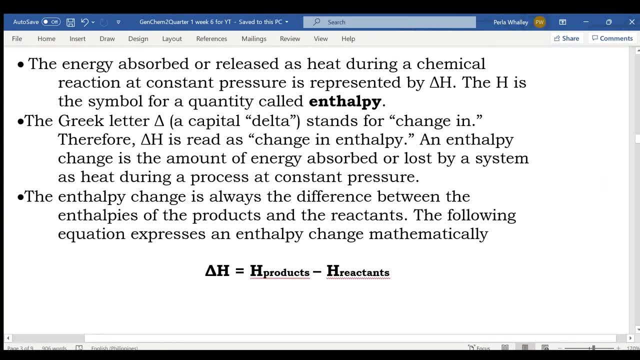 reactants. the following expression expresses an enthalpy change. mathematically, change in enthalpy is equal to enthalpy of the products minus enthalpy of the reactants, or is equal to the energy of the products minus the energy of the reactants. 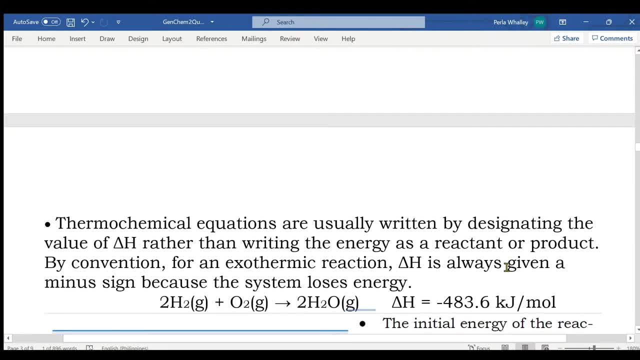 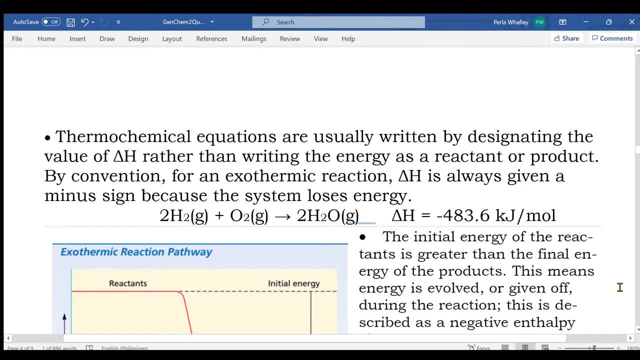 thermochemical equations are usually written by designating the value of Delta H rather than writing the energy as a reactant or product. by convention for an exothermic reaction, Delta H is always given a minus sign because the system losses energy. so here it is negative when it. 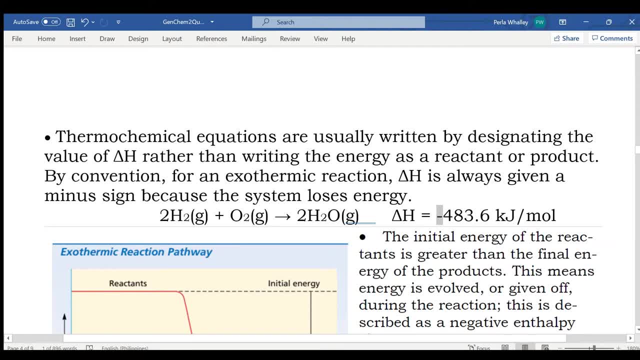 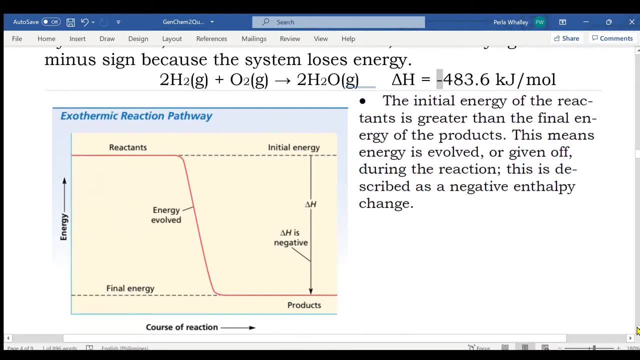 is negative, that means it is negative, so it's negative. in that case it is negative. but if you an exothermic reaction and the system loses energy during the reaction, by looking at this graph, this figure, so here this is energy and here is the course of reaction. this is the x-axis and this 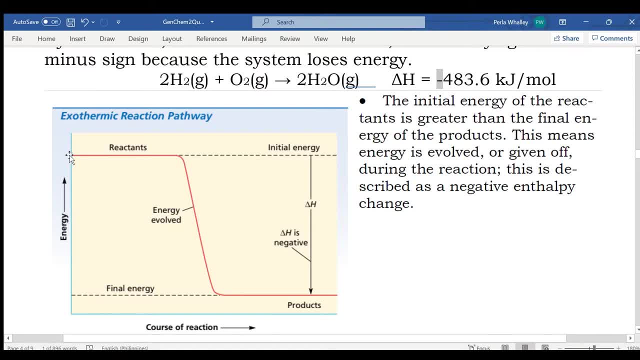 is the y-axis, so the energy of the reactants is higher compared to the energy of the products, which is here. so during the reaction that means the energy was released, resulting to the lesser energy of the products. so the delta H is negative for an endothermic reaction delta. 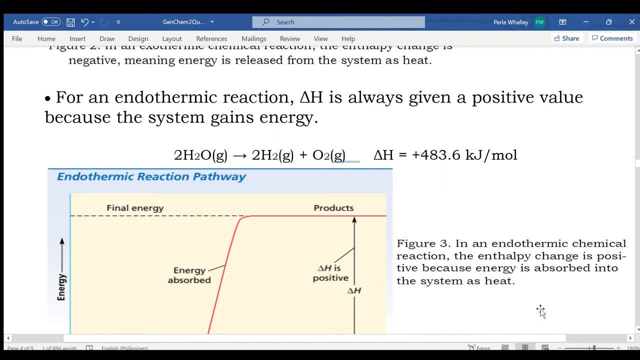 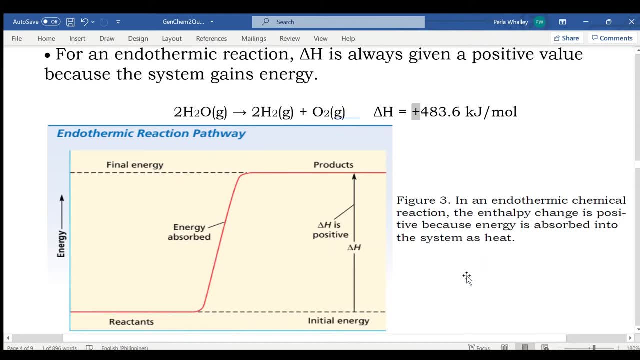 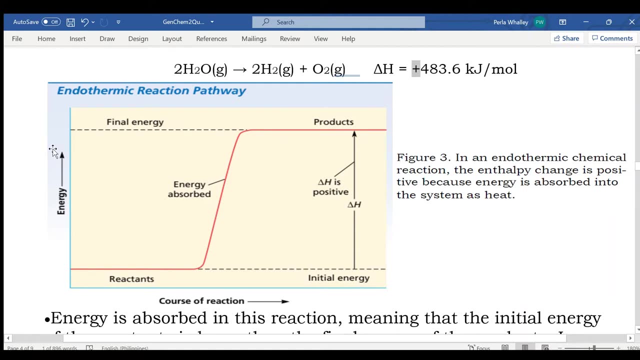 H is always given a positive value because the system gains energy. it's here positive. looking at this figure- energy y-axis and the course of our reaction x-axis- at the start the energy of the reactants is low. during the reaction it increases and it ended that the products have higher energy compared to the reactants. that is why 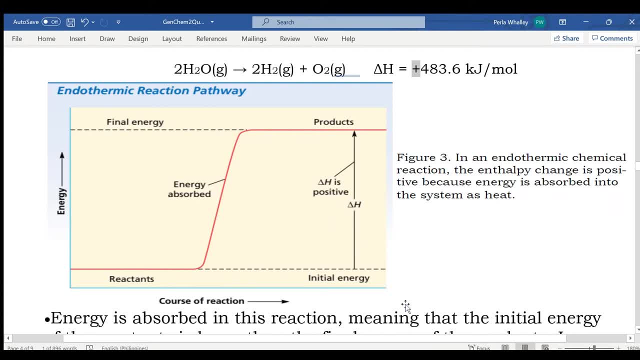 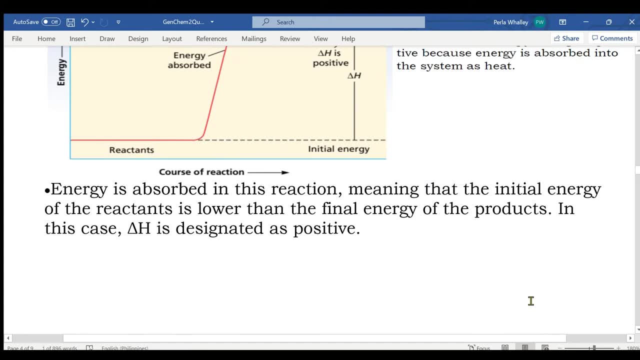 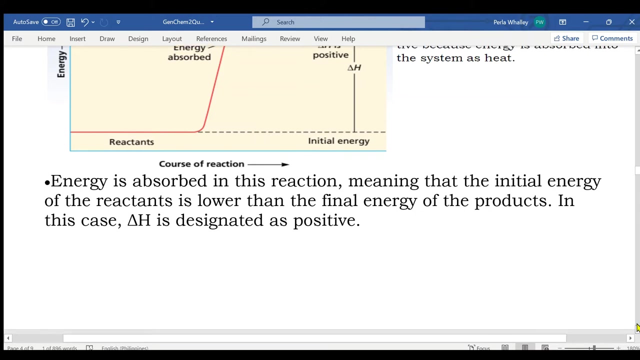 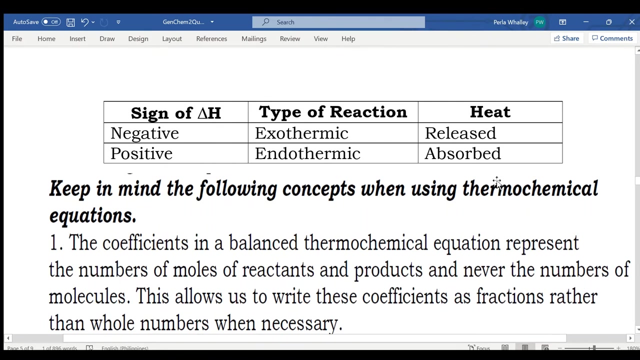 the delta H is positive, energy is absorbed in this reaction, meaning that the initial energy of the reactants is lower than the final energy of the products, in case, in this case, delta H is positive. so we have a table to summarize: sign of delta H. if it is negative, the type of reaction. 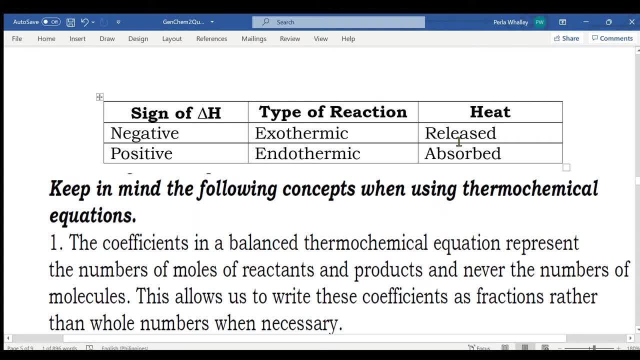 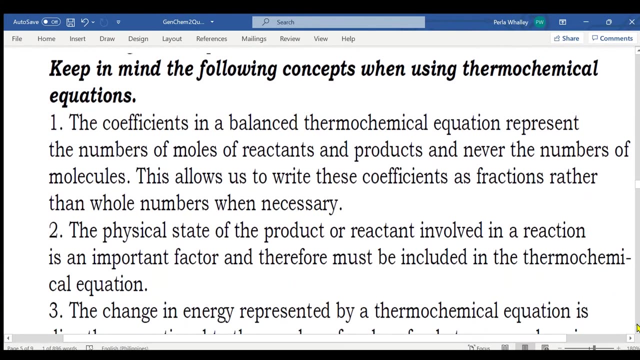 is exothermic. that means heat is released when the delta H is positive. the type of reaction is endothermic and the heat is absorbed by the system, by the system. keep in mind the following concepts when using thermochemical equations: the coefficients in a balanced thermochemical equation represents the number of moles, of reactants and products, and 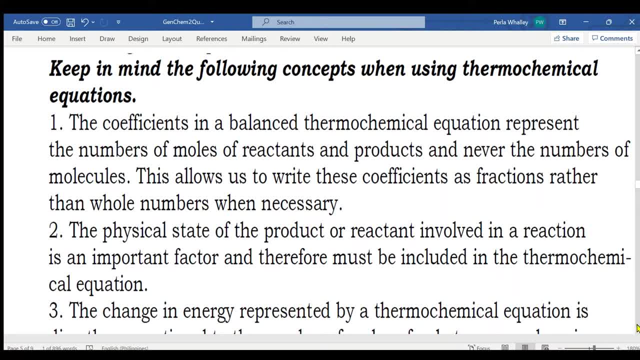 never the number of molecules. this allows us to write this coefficients as fractions rather than whole numbers, when necessary. the physical state of the product or reactant involved in a reaction is an important factor and therefore must be included in the thermochemical equation. physical states such as gas, solid liquid. 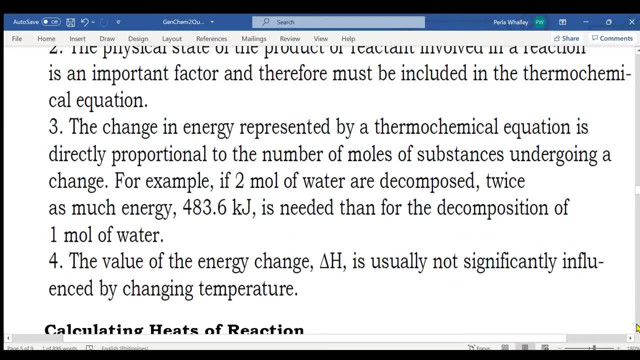 the change in energy represented by a thermochemical equation is directly proportional to the number of moles of substances undergoing a change. for example, if two moles of water are decomposed, twice as much energy- 4.83.6 kilojoules- is needed than for the decomposition of one mole of 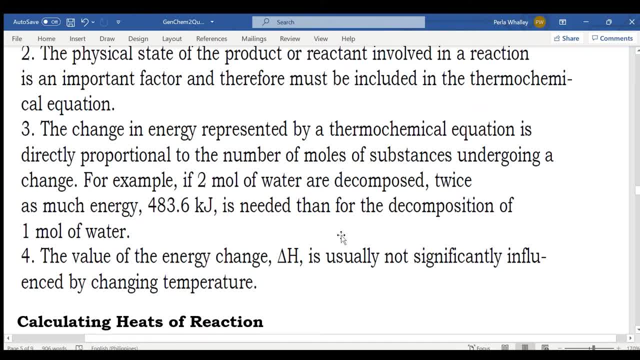 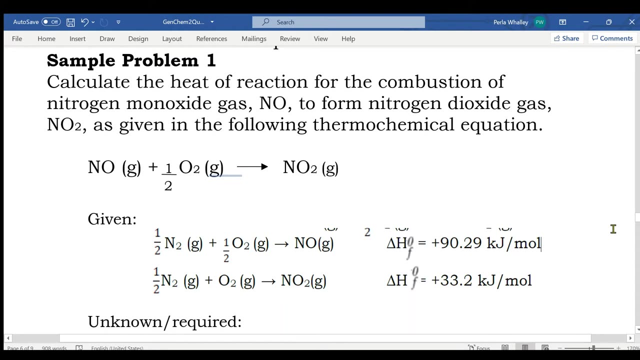 water. so to decompose two moles of water, we multiply 483.6 times two, which is equal to 967.2 kilojoules. sample problem number one: calculate the heat of reaction for the combustion of nitrogen monoxide gas and O2. form: nitrogen dioxide gas and O2 as given in the following thermochemical equation: 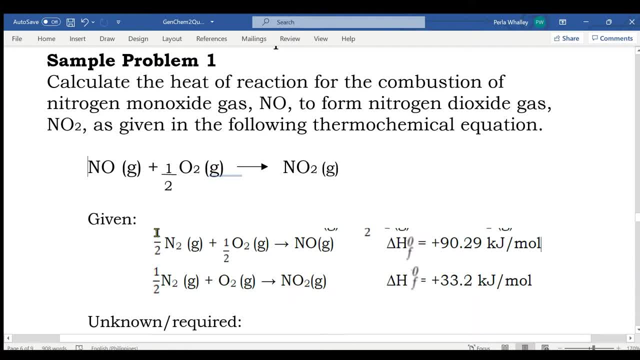 so this is our equation and we have the given. this is the equation that we need to look for, the required equation. so we have the given. one half mole of nitrogen gas plus one half mole of oxygen gas forms one mole of nitrogen oxide gas, which has a standard heat of formation. 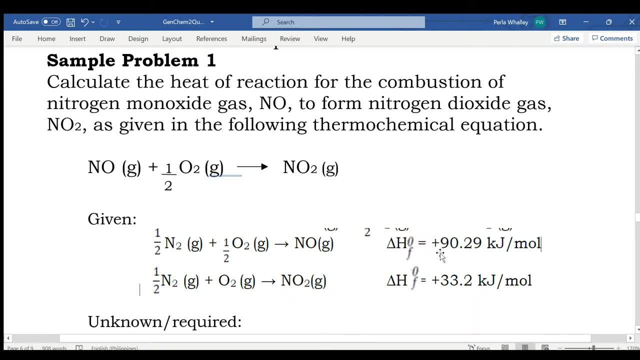 of positive ninety point two, nine kilojoules per mole. the second equation is: one half mole of nitrogen gas plus one mole of oxygen gas forms one mole of one of nitrogen dioxide gas, with the standard heat of formation of positive thirty three point two kilojoules per mole. 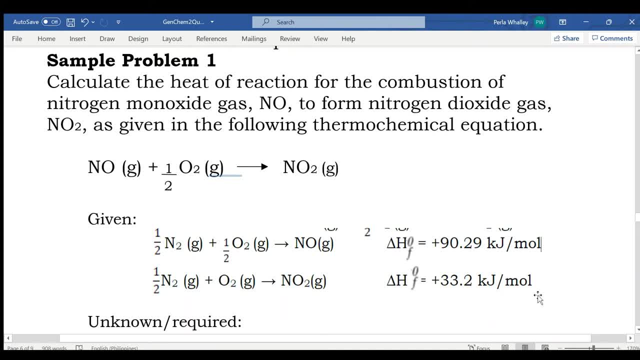 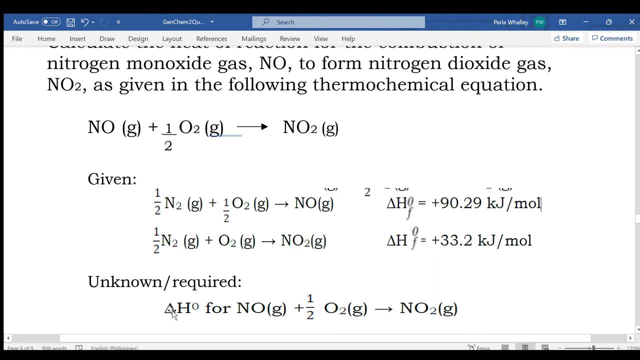 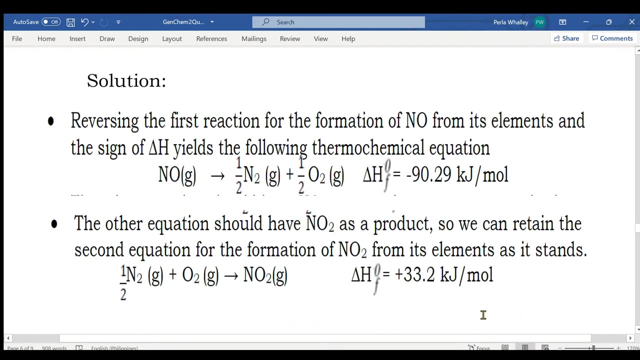 then we have the unknown. this is standard enthalpy of reaction. Delta H: zero for the equation for this equation. so the solution reversing the first reaction for the formation of an O from its elements and the sign of Delta H yields the following thermochemical react equation: so the first equation was reversed. 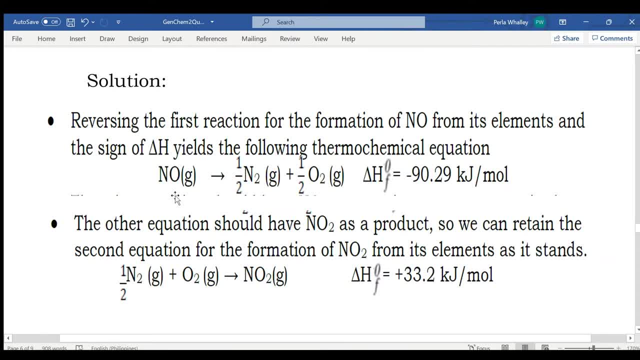 when the equation is reversed, that means the sign is also reversed. so we have now an O gas in the reactant side and one half mole of nitrogen gas, plus one half mole of oxygen gas and the product side. the other equation should have nitrogen dioxide as a product, so we can retain the second equation for 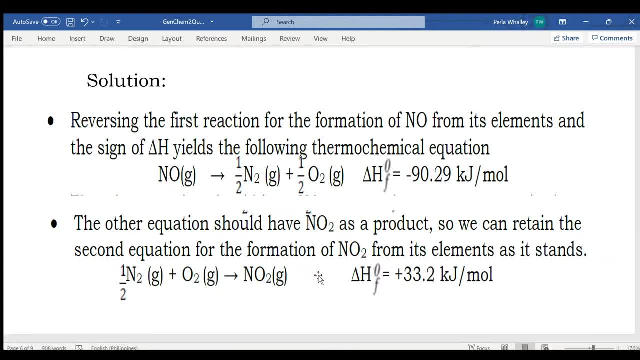 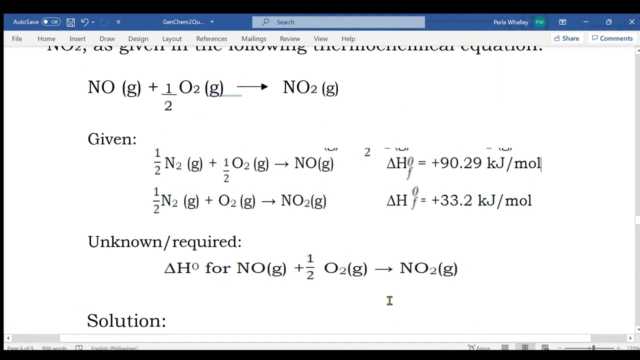 the formation of nitrogen dioxide from its elements as it stands. so we have one half mole of nitrogen gas plus one mole of oxygen gas forms one mole of nitrogen dioxide gas. okay, and then we have the standard heat of formation is still positive because it was not reversed. now let's go back here. why do we need to reverse the first? 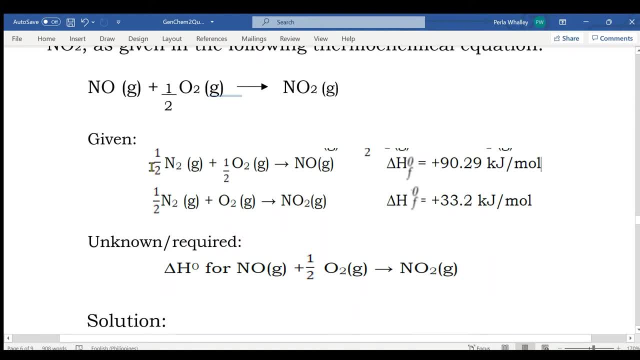 equation and why is it that the second equation has stayed as is? so the required equation is: the native nitrogen oxide gas should be- and the reactant side and also one-half mole of the oxygen gas. so we need nitrogen oxide and of reactant side. ok, so we need to reverse. 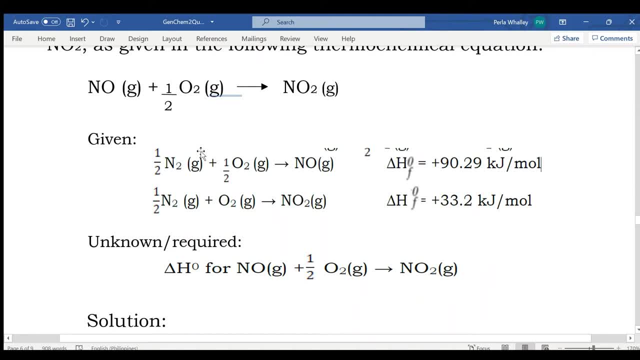 it so that we could have nitrogen oxide and the product, or in the reactant side. and then why we did not reverse the second equation? it's because we need the nitrogen dioxide gas in the product. so we will not reverse the equation. and remember that if we reverse the equation, the sign will also reverse, so this: 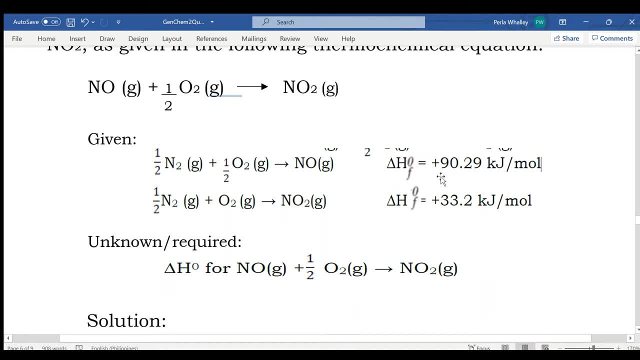 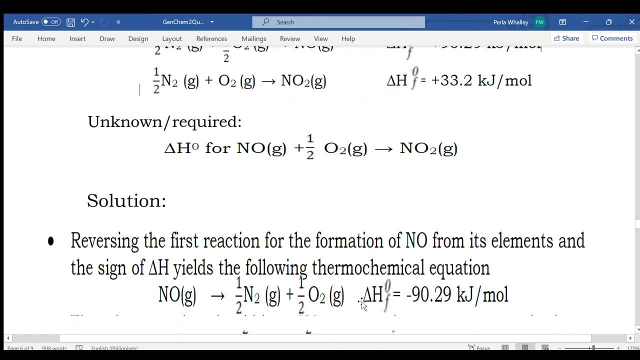 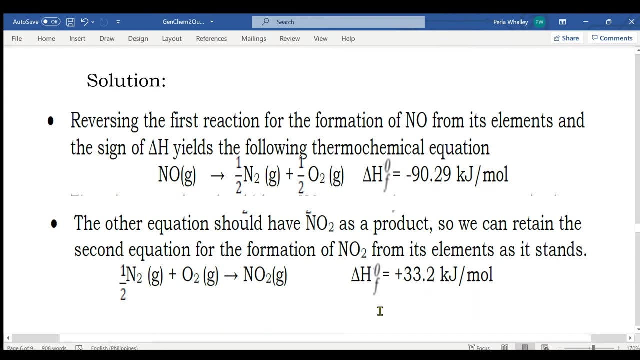 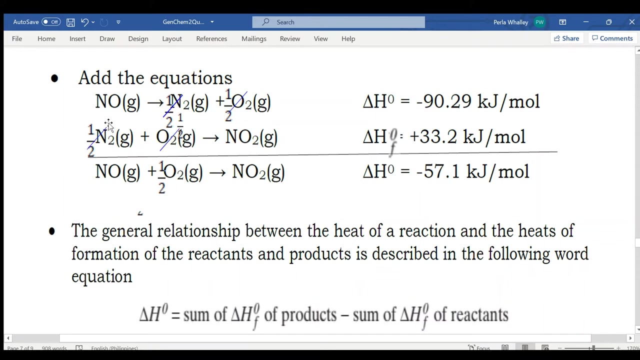 is positive, so when we reverse it, the sign will become negative. so that's happened here. okay, it becomes negative because we reversed equation number one and equation number two stays the same. positive because it we did not reverse. now we add the equations. so when we add the equation, we cancel out substances. 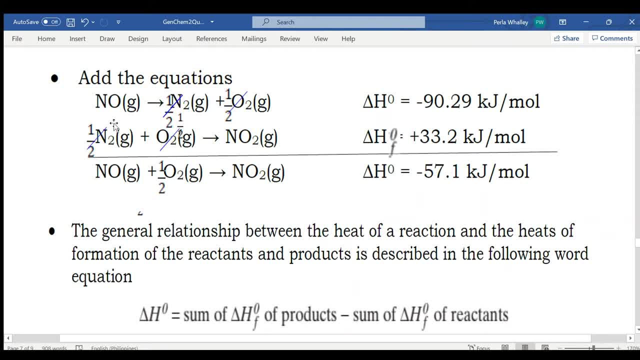 that are similar. so we cancel out substances that are similar between the two equations. but the cancellation would be on the product and reactant, product and reactant or reactant and the product. so let's see nitrogen oxide. is it canceled with nitrogen dioxide? no, because those two 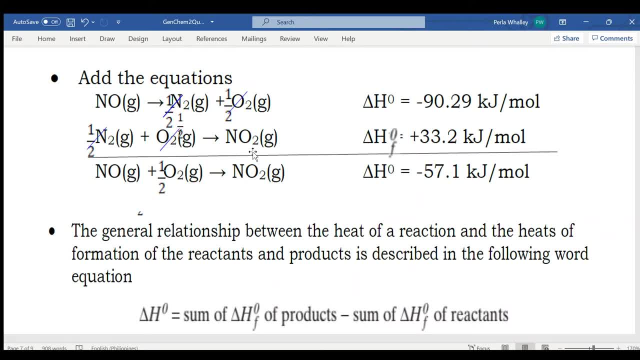 substances are different. so let's go to the product. we'll check if it has similar substance with the reactant of the equation number two. so one half and two, one half and two, that means this two are canceled. and then one half oh two and then we have one Oh two. so when half auto canceled but we still 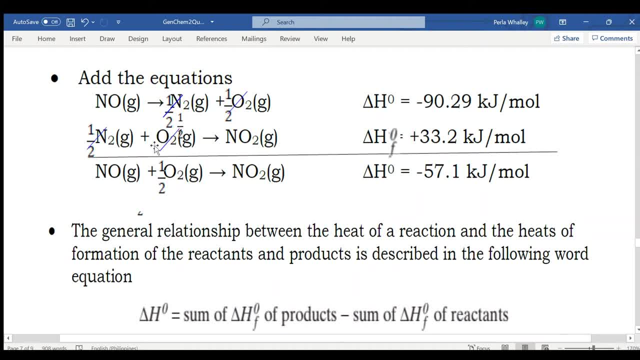 have remaining one half auto here, so we have to write all the remaining substances in the reactant side. okay, then we have NO gas. plus, we have a remaining 1 half mole of O2 gas and that's, there's nothing more. so we have to write here. 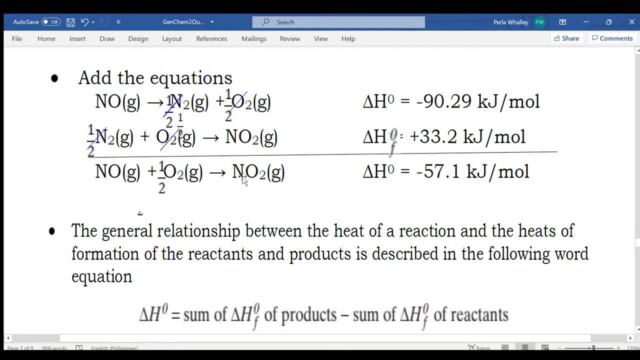 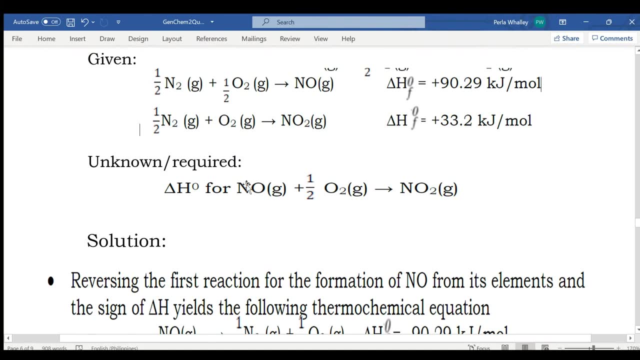 the RO, and then we'll go to the product side. the product side. here we only have and O2, okay, so this is now the equation that is required. this is the one here. okay, this is the one. so we got that, and then what we will do now is also again. 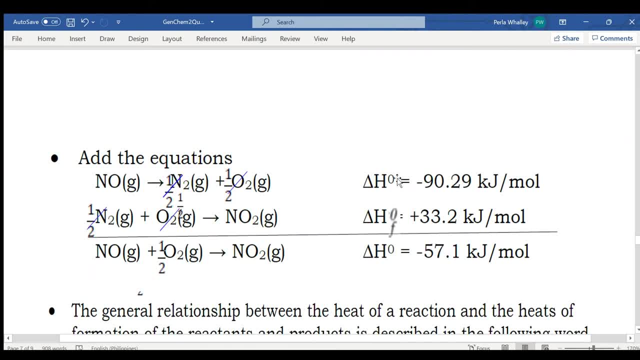 add this heat of formation. so minus 90 plus- I'm not minus 90 point two- nine kilojoules per minute mole plus thirty three point two kilojoules per mole is equal to fifty seven point one kilojoules per mole. the sign is carried over, but by the number. 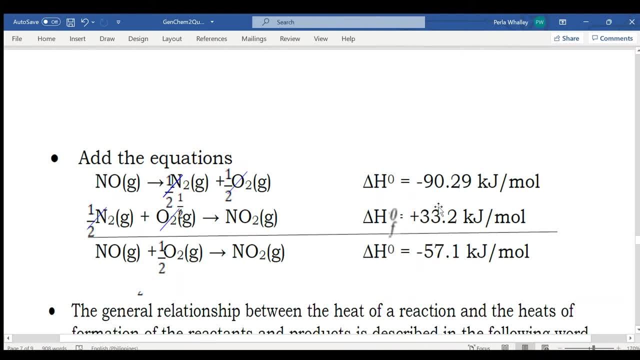 with a bigger value. so the number with a bigger value here is 90 and the sign is negative. so that is why the answer will also have a negative sign: you. so that means this equation, thermal chemical equation, is exothermic because the Delta H is negative. so if you notice that there is no F here in the symbol, so 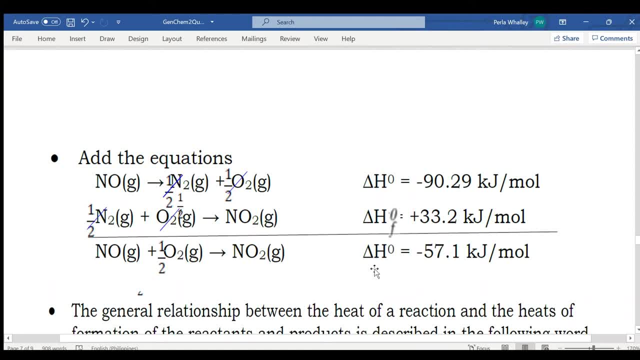 that means this is what we call the standard enthalpy of reaction, and this is now. this is here the standard heat of formation. this one here only is lacking an F. okay, so the answer here is standard enthalpy of reaction, which is equal to minus fifty seven point one kilojoules per mole. the 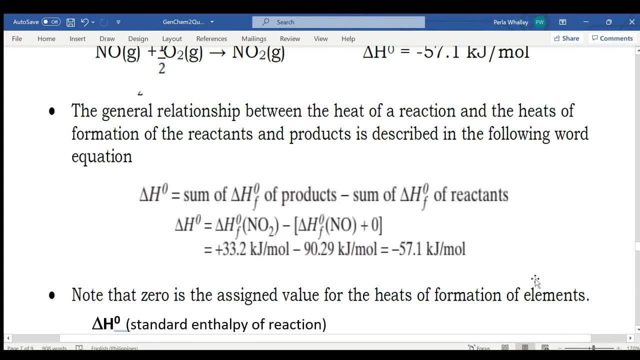 general relationship between the heat of reaction and the heats of formation of the reactants and products, as described in the following word equation: the standard enthalpy of reaction is equal to the summation of the standard standard heat of formation of the products minus the summation of the standard heat of. 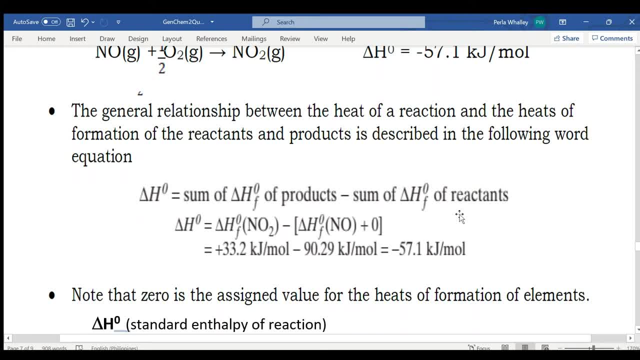 formation of the reactants. okay, so we just have to substitute the given data to the formula. so summation of the products here: thirty three point two kilojoules per mole, minus that of the reactants, it is ninety point two. nine kilojoules per mole is equal to fifty seven point one. 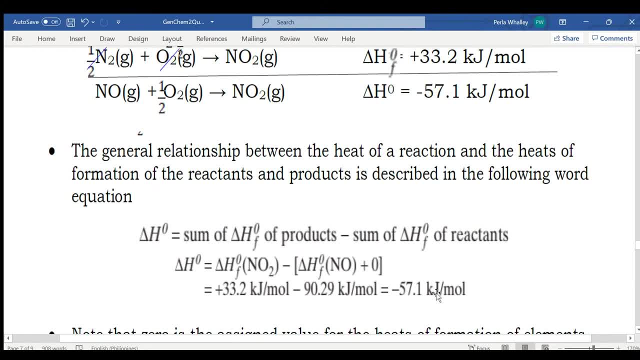 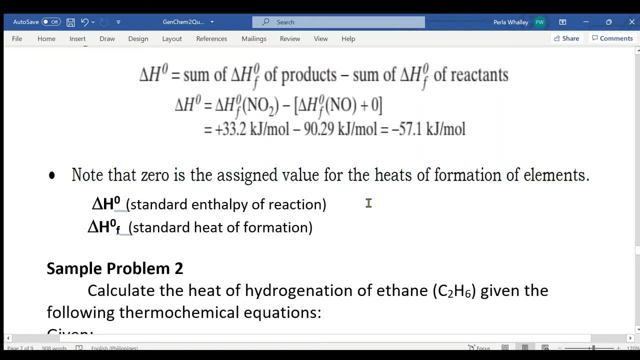 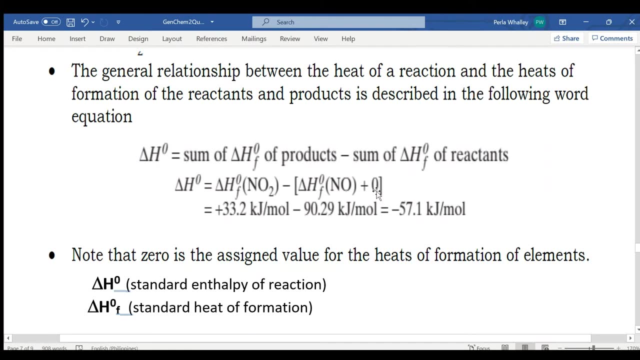 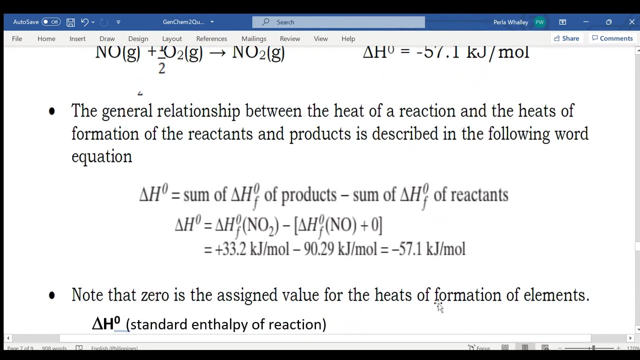 kilojoules per mole, which is equal. note that zero is a sin value for the heats of formation of elements. so here this is zero, because in the reaction, the reactant, we have oxygen. okay, that is an element. so note that the Z, that zero, is the assigned value for the heats of formation of elements. and again, Delta H. 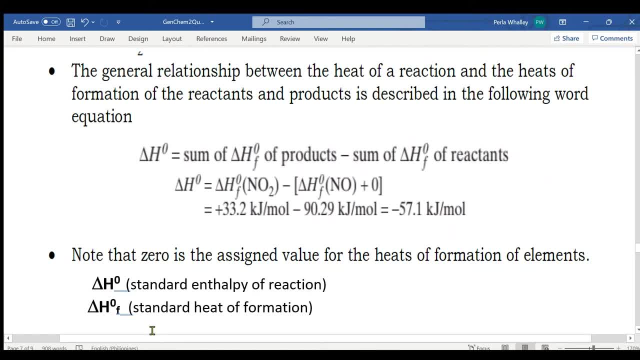 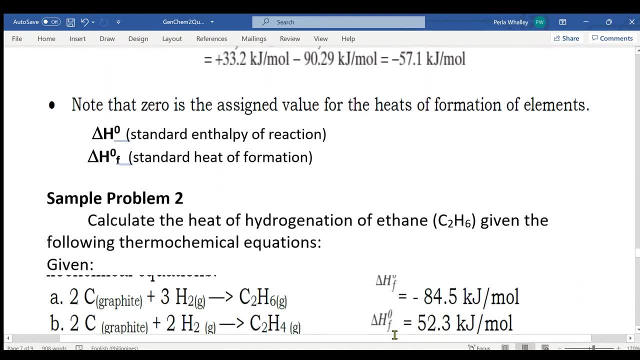 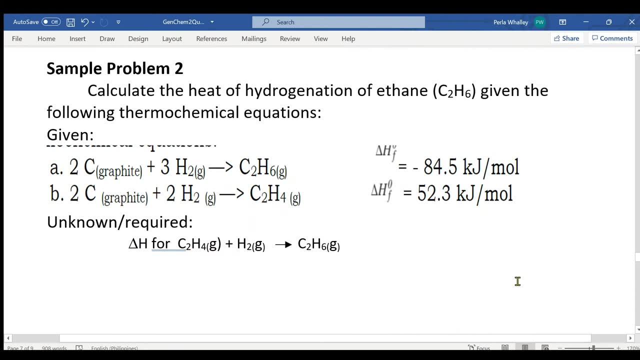 zero standard enthalpy of reaction and Delta H, zero F standard heat of formation. let's go to problem number two: calculate the heat of hydrogenation of the same, given the following thermochemical equations: so we have two moles of graphite or carbon plus three moles of hydrogen. class forms one mole. 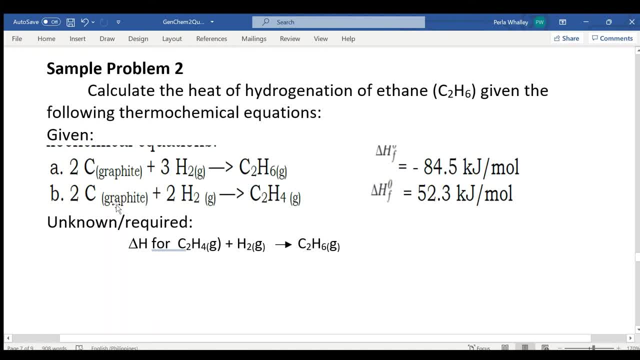 of a thing. there'll be two moles of graphite plus two moles of hydrogen. cause forms one mole of a thin, and this are the corresponding standard. heat of formation. unknown order required is the Delta H for this form of equation. okay, and also we need to get this equation at the end because this is the 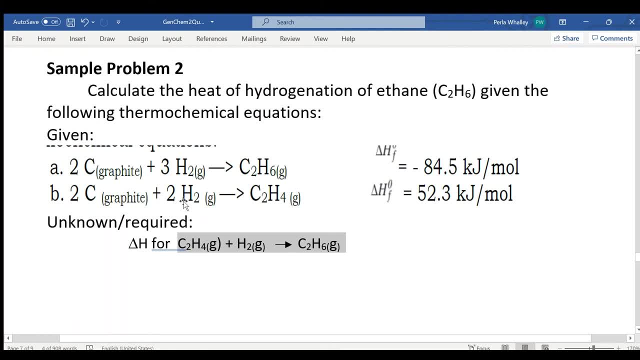 required equation from these two equations. so, looking at this class, you can see that C 2 H 4 should be in the reactant side. that means this would be what reversed and C 2 H 6 is in the product side, so there is no need for it to be reversed. 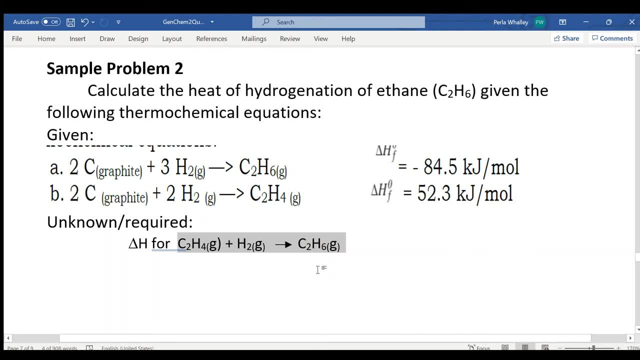 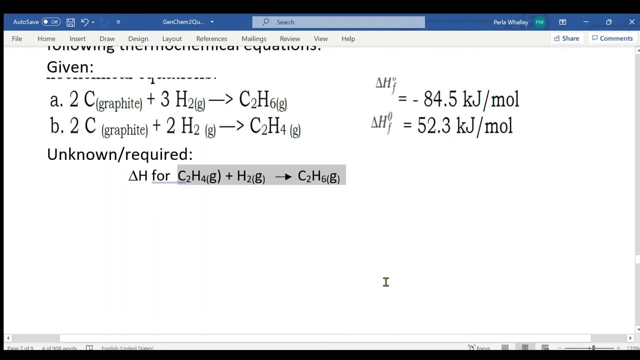 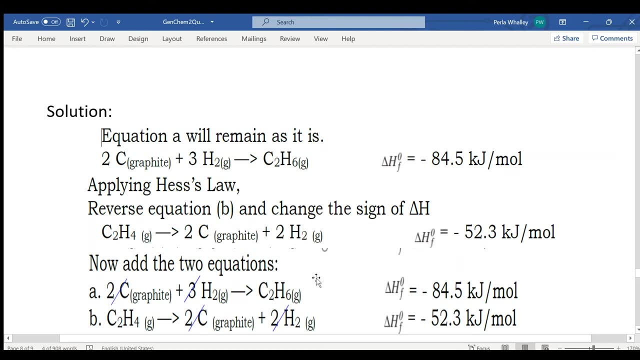 it will stay as is. so this is positive here and this is negative solution. equation: equation a: you will remain as it is. applying. has flow reversed. equation B and change the sign of Delta H. so C 2 H for gas forms two moles of carbon plus two moles of hydrogen gas and it becomes 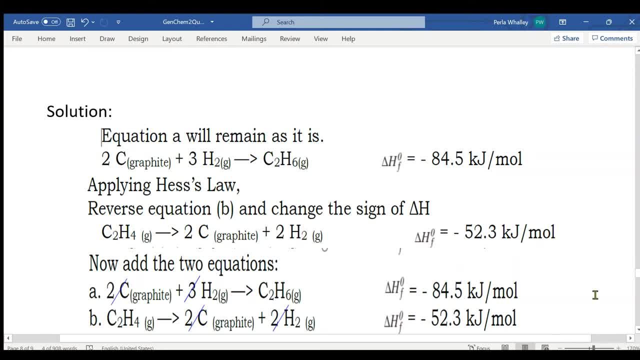 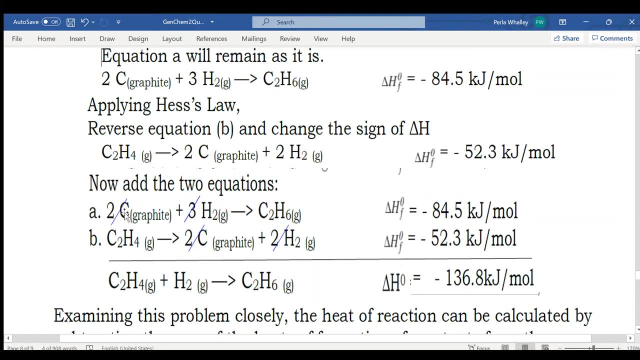 negative. now we are the two equations. so we have the reactant and we look at the product side of the other equation, if we can cancel similar substances, so to graphite, to graphite cancel. 3h2 is cancelled with 2h2 here, but so we still have one hydrogen remaining here, one hydrogen gas, and then the product and 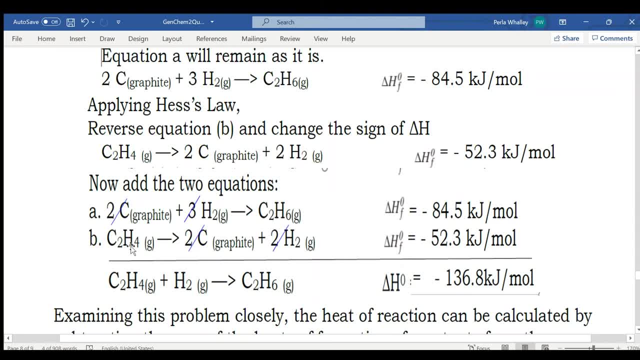 the reactant there is. there is no similar substance, so we have to. it have to remain as is now. we will copy the remaining substances, the reactant side. so we have H 2, yes, and we have C 2, H 4. if you write H 2 first, it is okay, but the 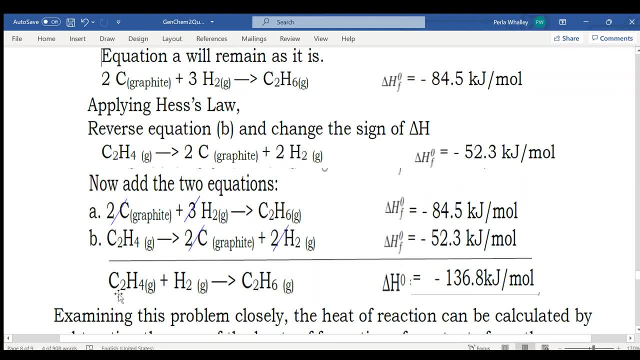 correct or the best answer would be C 2 H 4. you write C 2 H 4 first and copy the gas. the state plus 1 mole of H 2 gas will form 1 mole of C 2 H 6 gas. now we add this up so because they have. 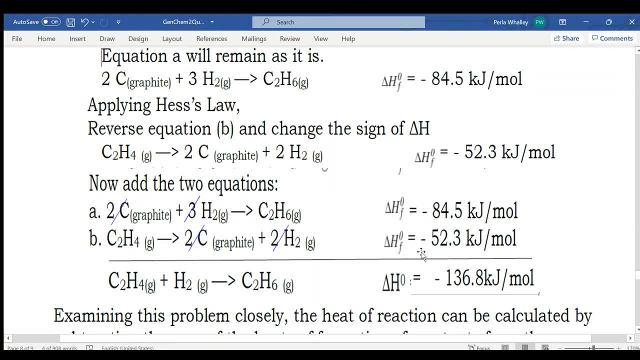 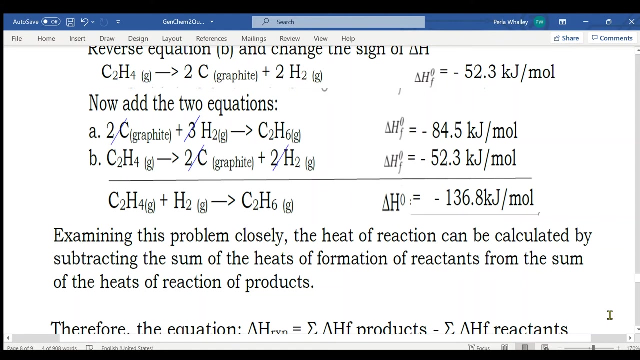 similar signs. the symbol will be easy. it is also negative. we add it up, so the answer is 136 point 8 kilojoules per mole. so the standard enthalpy of reaction of this equation is this. examining this problem closely, the hit of reaction can be calculated by subtracting the sum of the 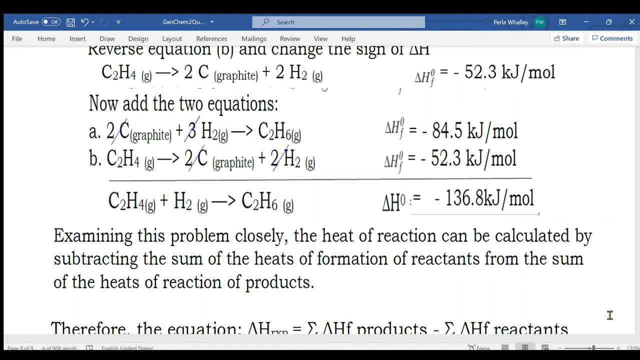 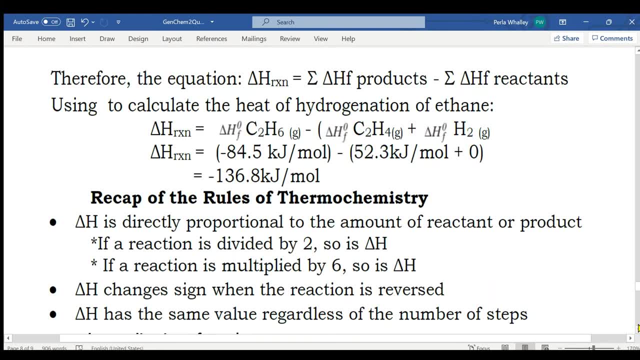 hits of formation of reactants from the sum of the hits of reaction of the products. therefore, the equation, the standard enthalpy of reaction is equal to the summation of the standard hit of formation of the products minus the summation of the standard hit of formation. 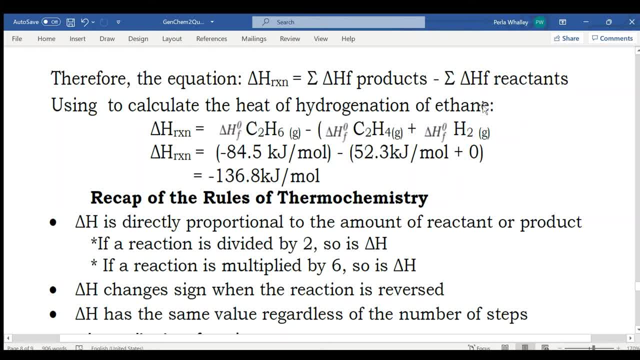 of the reactants. using to calculate the hit of hydrogenation of a thing is equal to you minus 84.5 kilojoules per mole. minus 52.3 kilojoules per mole, that is for C2H4 plus H2, which is 0 for elements, the answer is equal to negative 136.8 kilojoules per mole. 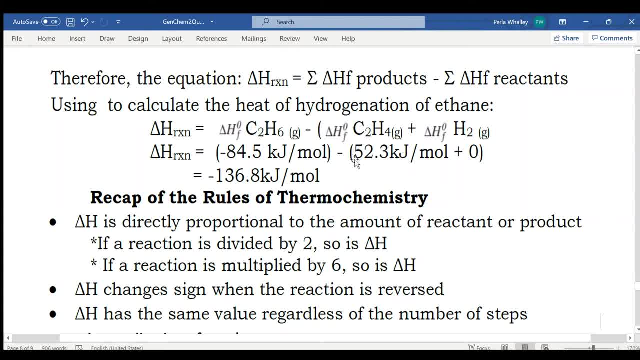 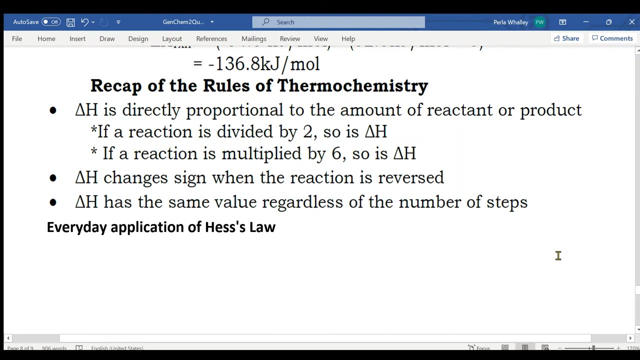 so when subtracting you need to change the sign here to negative and then proceed to addition. that is why the answer is negative: 136.8 kilojoules per mole. recap of the rules of thermochemistry: delta H is directly proportional to the amount of. 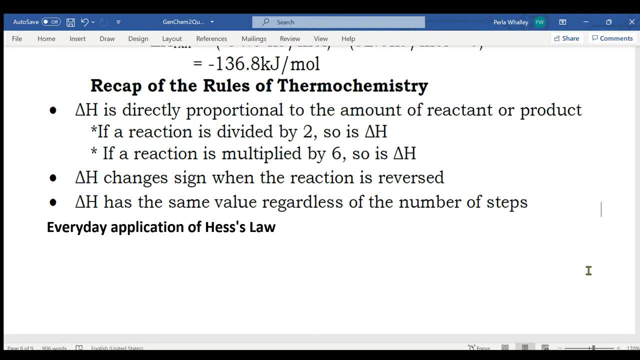 reactant or product. if a reaction is divided by two, so is delta H. if a reaction is multiplied by six, so is delta H. delta H changes sign. when the reaction is reversed, delta H has the same value, regardless of the number of steps. now let's go to everyday application of Hess's law. 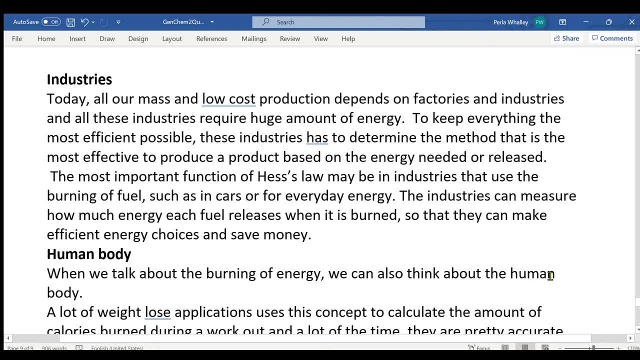 industries. today, all our mass and log cost production depends on factories and industries, and all this industries require huge amount of energy to keep everything the most efficient possible. this industries has to determine the method that is the most effective to produce a product based on the energy needed or released. the most important function of his law may be in industries. 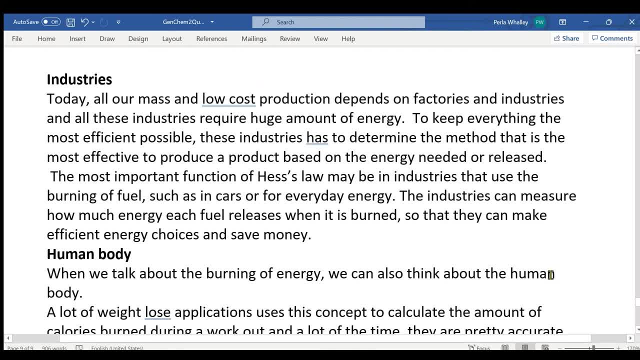 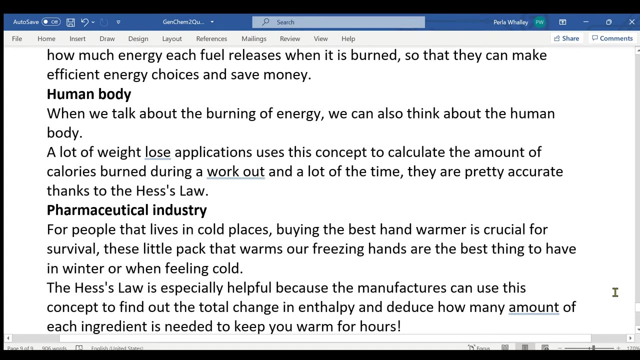 that choose the burning of fuel, such as in cars for or for everyday energy. the industries can measure how much energy its fuel releases, energy is burned, so that they can make efficient energy choices and make and save money the human body. when we talk about the burning of energy, we can also think: 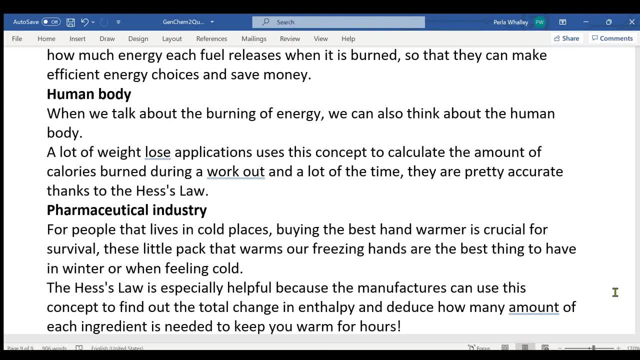 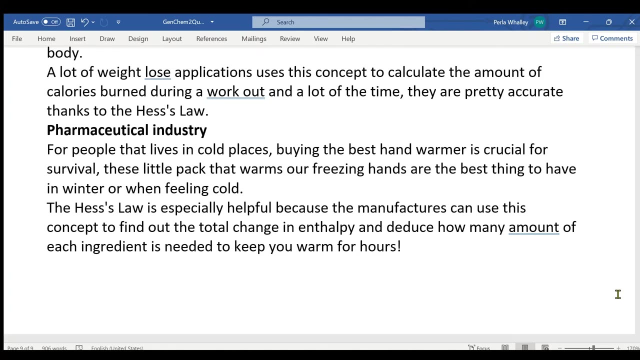 about the human body. a lot of weight loss application uses this concept to calculate the amount of calories burned during a workout and a lot of time of the time they are pretty accurate, thanks to the Hess's law pharmaceutical industry. for people that lives in cold places, buying the best hand warmer is crucial. 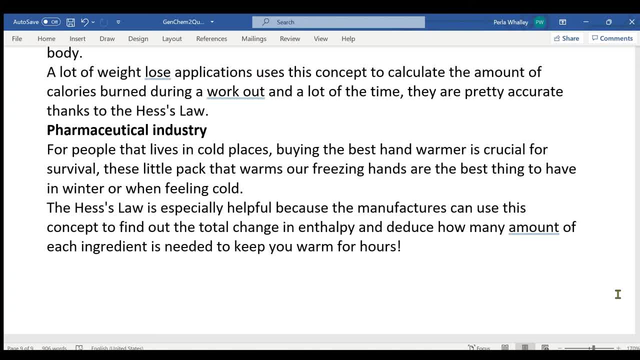 for survival. the little pack that warms our freezing hands are the best thing to have in winter or when feeling cold. the hess's law is especially helpful because the manufacturers can use this concept to find out the total change in enthalpy and the juice. how much energy is burned? 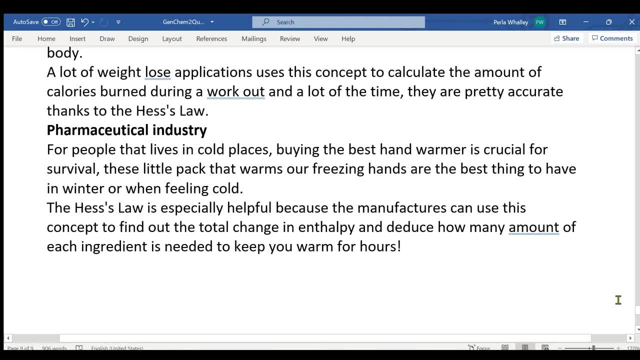 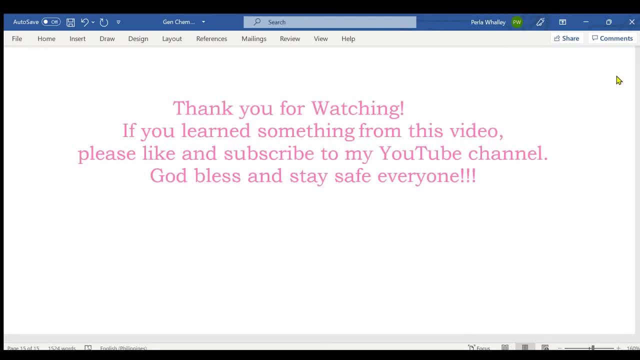 the hess's law is especially helpful because the manufacturers can use this concept to find out the total change in enthalpy and the juice, how much energy is burned, many amount of its ingredients is needed to keep you warm for hours. thank you for watching. if you learned something from this video. 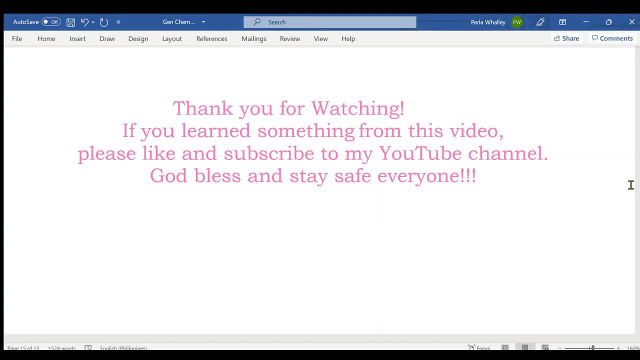 please like and subscribe to my youtube channel. god bless and stay safe everyone.